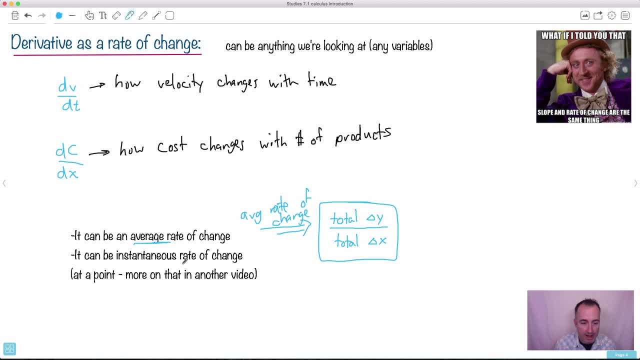 change, Or you can do it at a point, and we're going to do that in more detail. So I'm going to show you that. I'm going to show you that in sort of greater detail, But for right now it suffices to just. 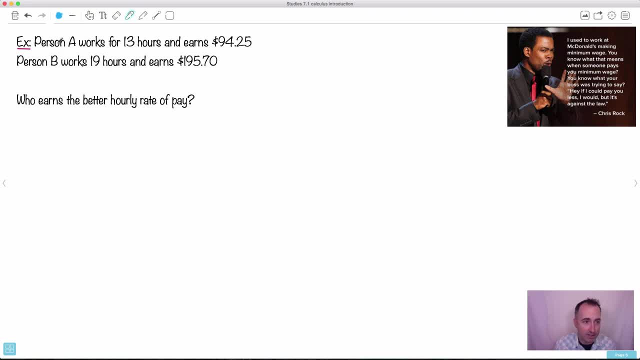 understand how this stuff right here works. Finally, we can do an example here. I mean, this is a really simple one. I like this joke from Chris Rock. He's basically saying he used to work at McDonald's getting a minimum wage. He said: you know what that is? It's like your. 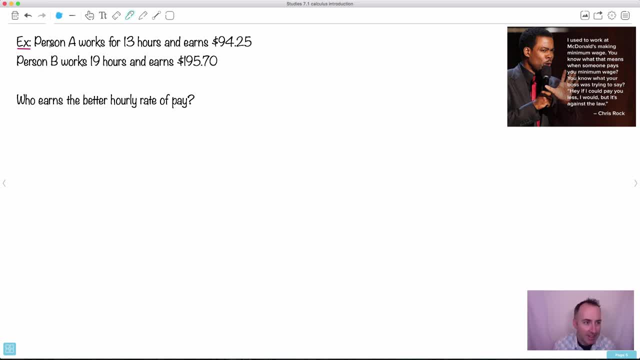 boss trying to say: hey, if I could pay you less I would, but it's against the law. Let's look at this rate of change here. You'll see this is actually a calculus question. You could see it that way: Person A works for 13 hours and earns $94.25.. Person B works for 19 hours and gets that. 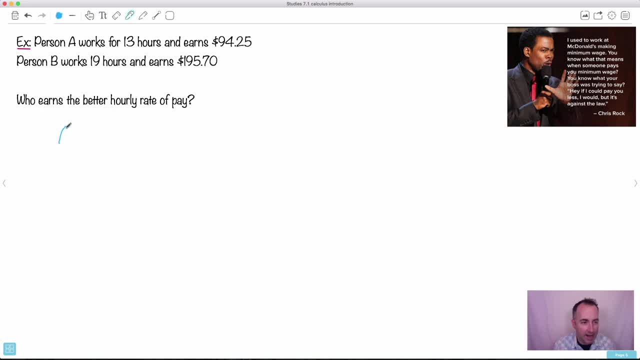 much. Who has the better hourly rate of pay. Watch this For A. I'm going to do an equation. I can call it dP like pay, dH for hours. See, like change in pay over change in hours. What's the? 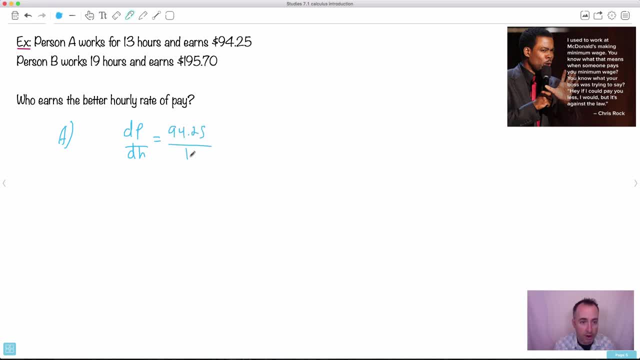 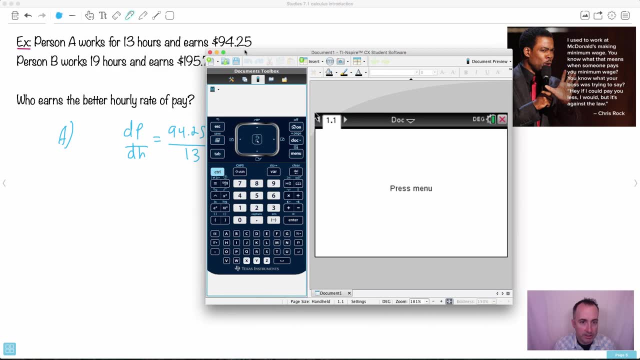 amount of pay they got, So 94.25 over the number of hours they worked, which is 13.. So that we can do. I'm just going to open up a calculator because I'm going to need that here, So let's actually. 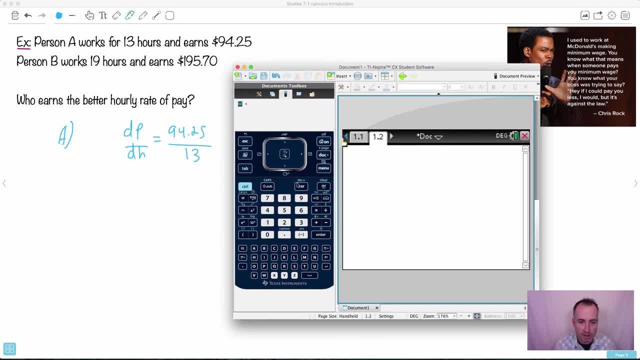 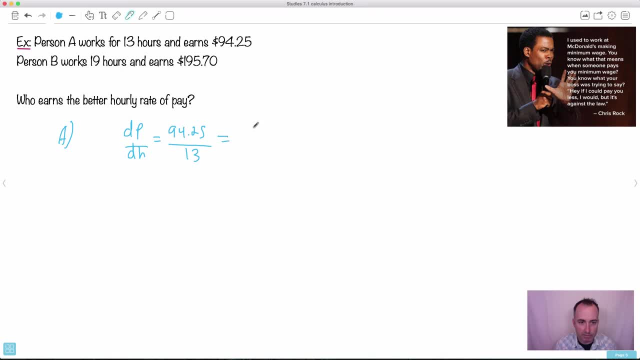 figure that out. It's a new page calculator, Let's just do that. So 94.25.. Divide that by 13 and I get 7.25,, for example. So that's dollars per hour. This could be this. 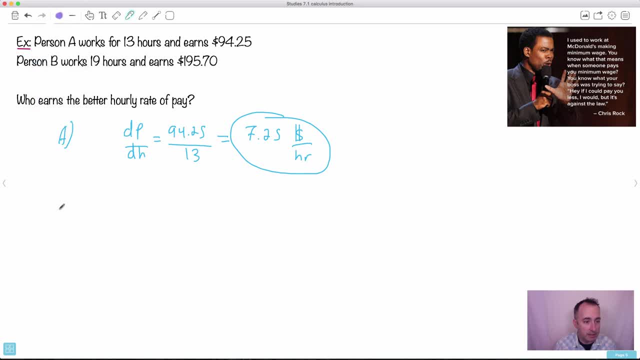 person's rate of pay. But then person B, let's just say they're dP, dH. I'm just trying to write it in calculus terminology. So change in pay over change in hour is going to be 195.70,. 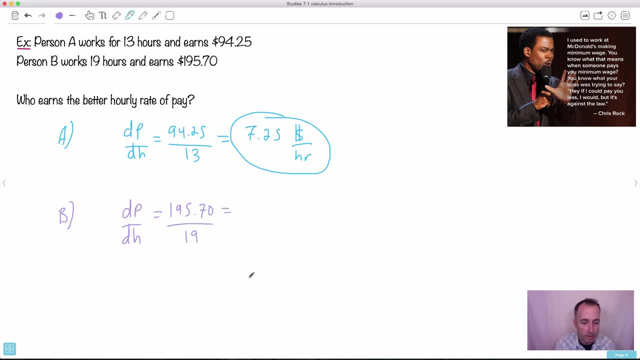 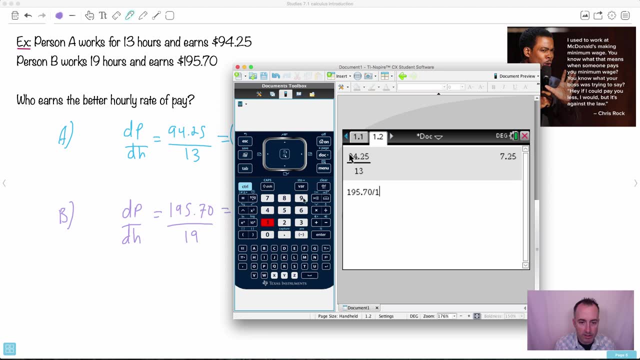 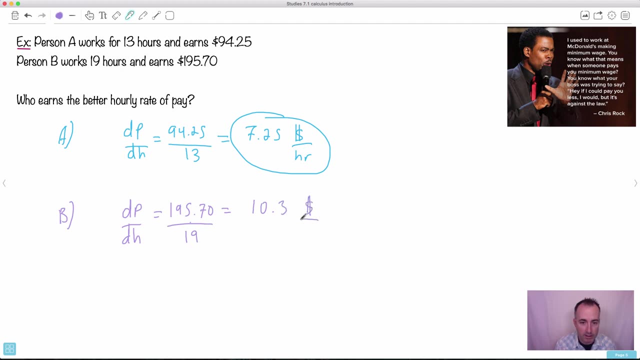 for example, over 13.. Oh sorry, 19 hours That will be. let's see what that is. This is basically how you can figure this out, right? So 70 over 19.. Let's figure out how much this person gets paid. This is 10.3.. So clearly this person. 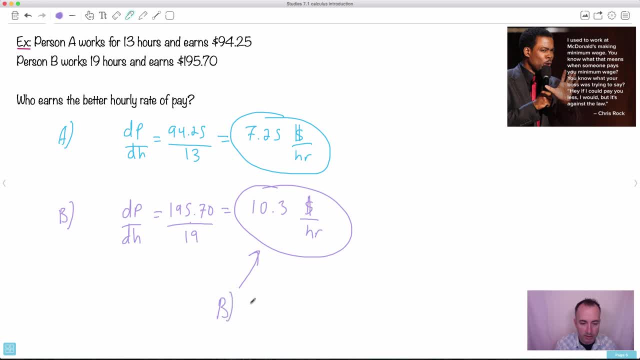 or your person B is the person you want to be, So person B earns the most. But the point of this here is just to introduce that. this concept of a rate of change is something you're familiar with. You've already heard of these things. with gradients of gravity: You've already heard of these things.